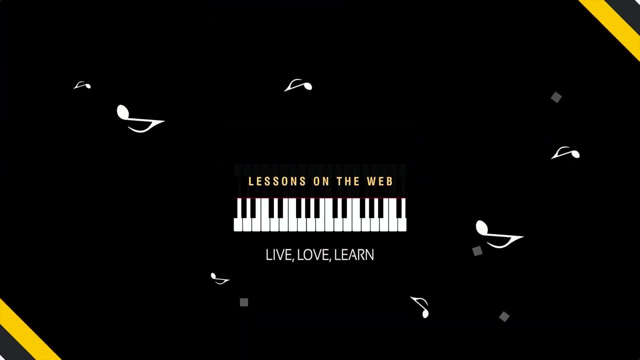 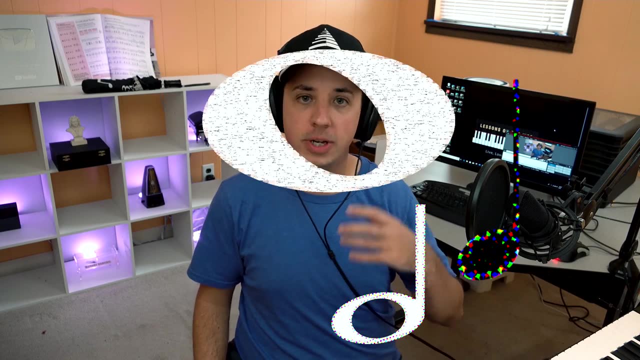 Let's get on to the lesson. The first thing you need to know about are simple note durations. These are quarter notes, half notes, whole notes, dotted quarter notes, maybe eighth notes, 16th notes, things like that, If you're not familiar with all that already, 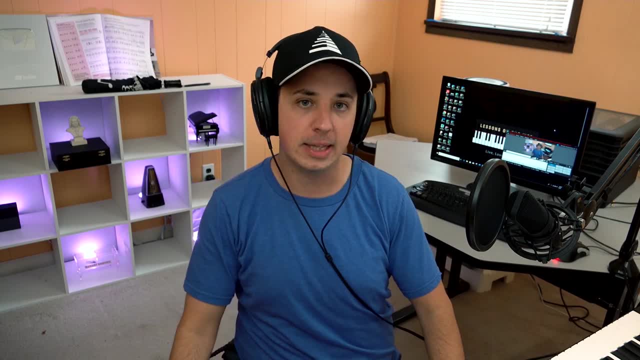 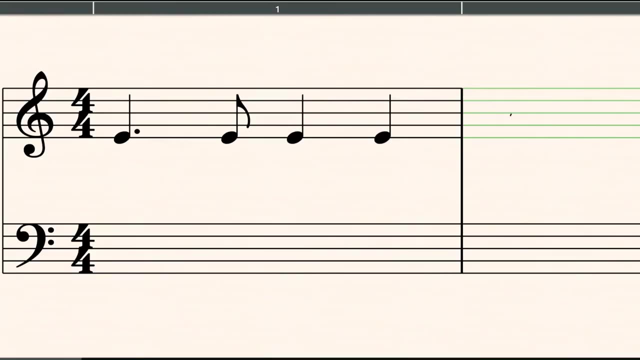 and how time signatures work and the whole thing. make sure you check out the link in the description because that will help you catch you up. All right on with the meat of the lesson. The first rhythm that students commonly get wrong is the dotted quarter and usually followed. 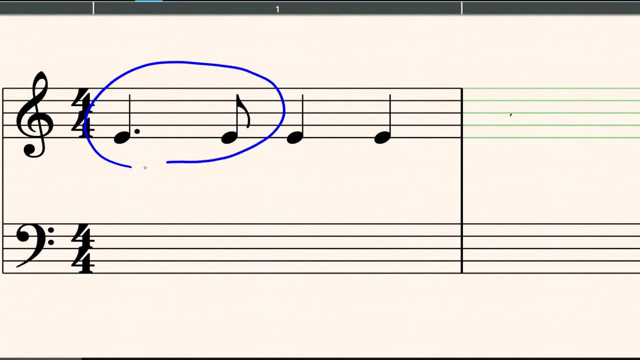 by an eighth rhythm. So we're really talking about from here to here. So let me show you how to do it. So hopefully you checked out that lesson I mentioned, or you know how to count already. So the thing is is obviously we're in 4-4 time signature. 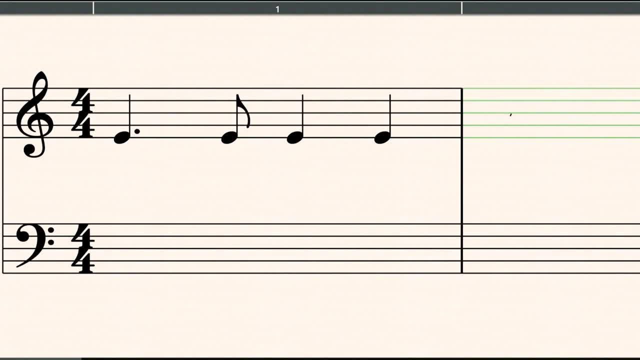 meaning we have four beats in a measure, So the total has to add up to four. So the thing is: is obviously beat, one is gonna hit there, So we need to figure out how long are we gonna be holding the dotted quarter for? Well, a dotted quarter note, as you might know. 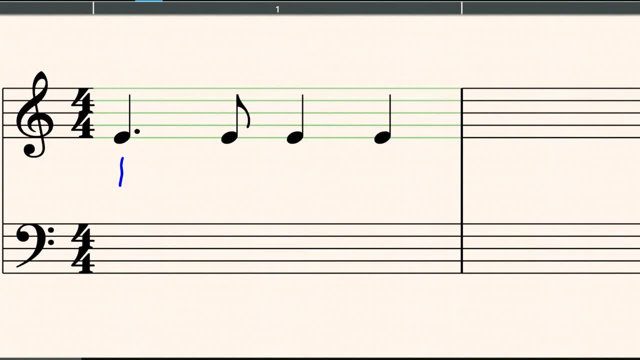 gets one and a half beats. And if you remember from when we were subdividing, let me write it over here so we can have our quarter note. That's right, Okay, so if you remember, with eighth notes we had to subdivide each beat. 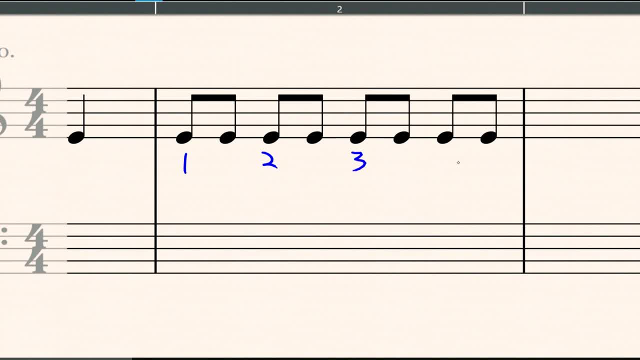 We still had our four beats: One, two, three, four. But to account for all these missing areas we had to come up with kind of a placeholder. So we used the term and It looks like a plus sign. So instead of one, two, three, four, 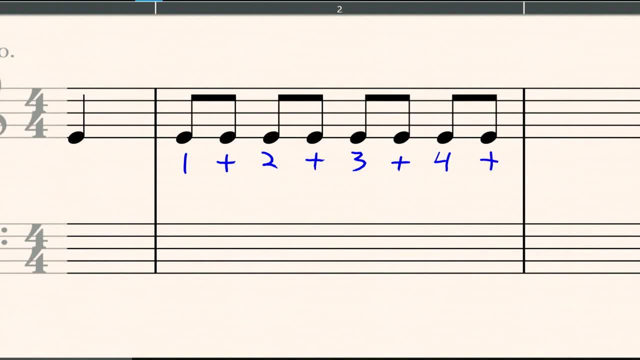 we count them twice as fast: One and two, and three and four, and The reason this is relevant is that each of these now represents half a beat. So there's half a beat on the number. There's another half a beat. There's another half a beat, half a beat. 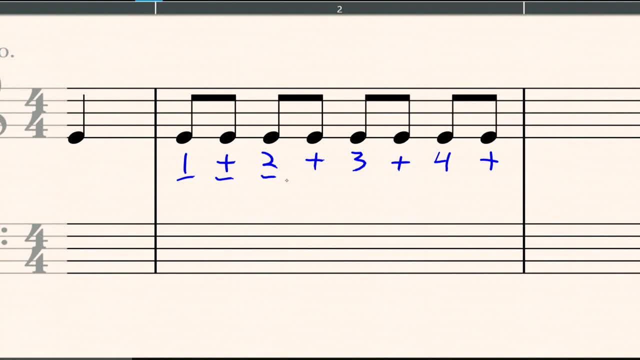 So just get in your mind that each of those- the one and the and two and the and- are each worth half of a beat on their own. Now the thing is is that I said the dotted quarter note is worth one and a half beats. 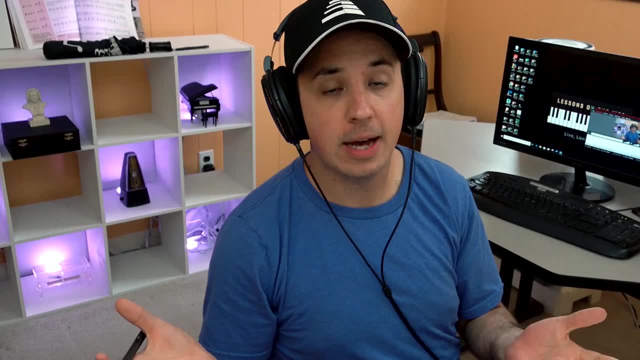 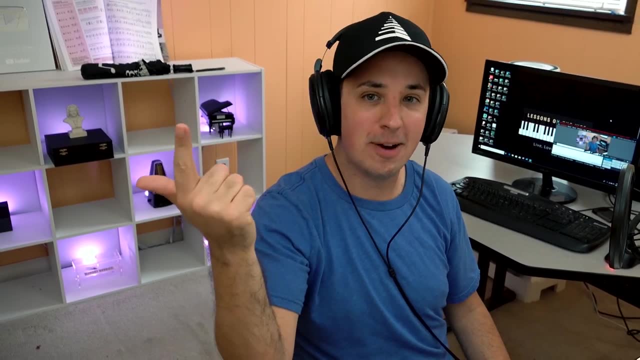 So the question I wanna ask you is how many halves in one and a half? Well, think about it: You have a half, So you have a half, then Plus another half, which is whole, So you have one, then Plus another half. 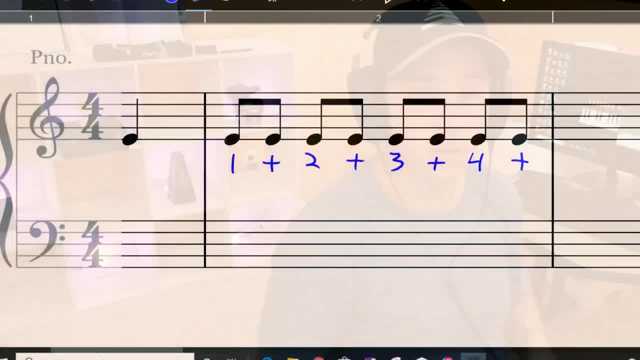 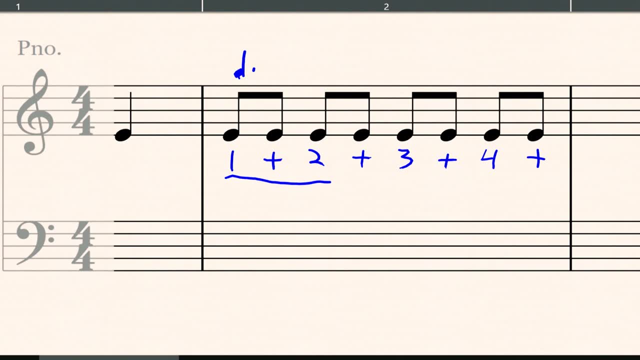 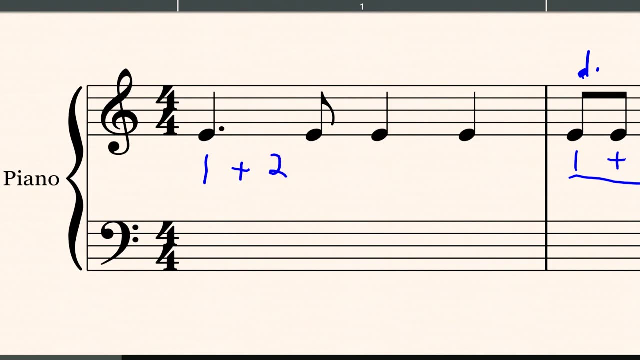 So you have three halves in one and a half. So, therefore, your dotted quarter note, which will look like this, should you remember, is gonna take up one and two. So here we go, We're gonna go back to our rhythm, and this is gonna take up one and two. 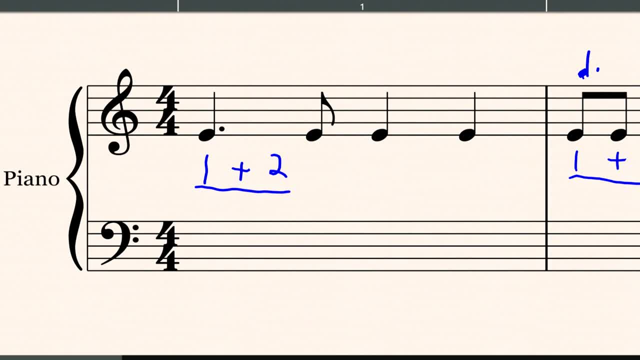 Just like that. I'm gonna draw a line underneath to indicate how long that's gonna be held for. The next eighth note is gonna be held on and, or pressed on and, And. then of course you have three, four. However, I do recommend you still count out the ands. 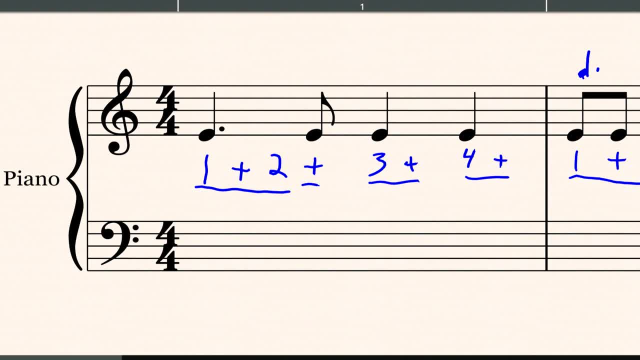 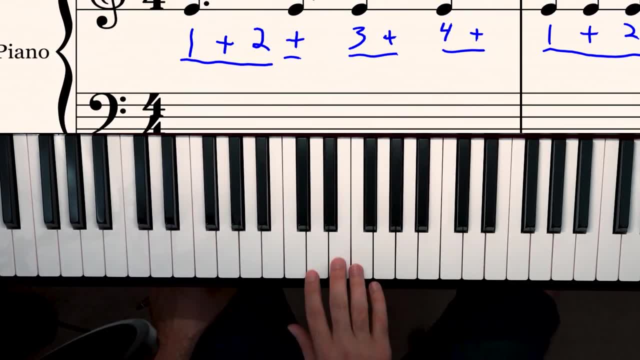 This is called subdivision, And the reason you do that, even though you're playing quarter notes, is to maintain a consistent tempo throughout. Let me show you how to play this now. So you go to your keyboard, obviously, And I'm gonna count it real slow. 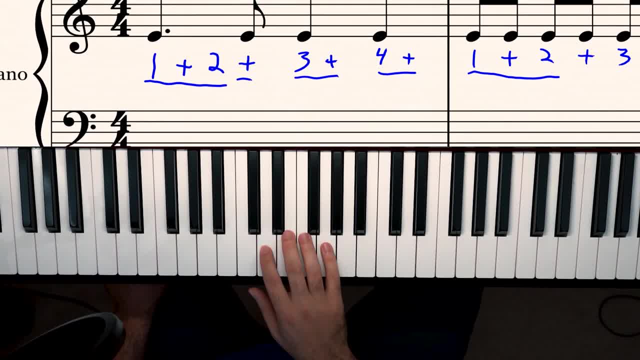 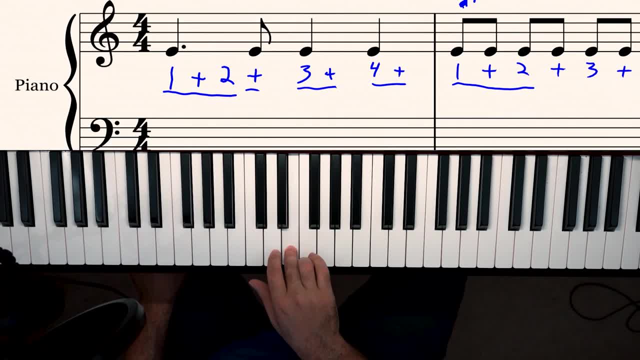 I'm just gonna be counting out the one and two and until I get to four Or the and of four. So here we go, One and two And three and four, and Obviously hitting each of those beats or each of those notes where they appear. 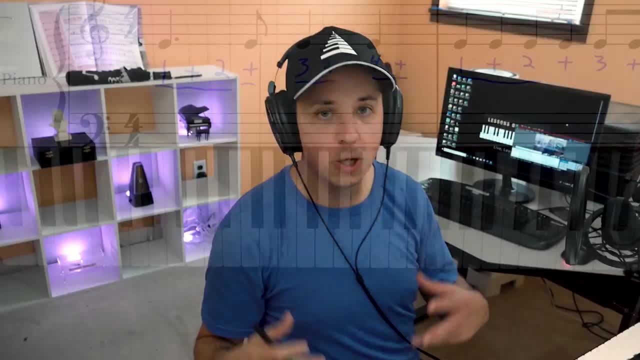 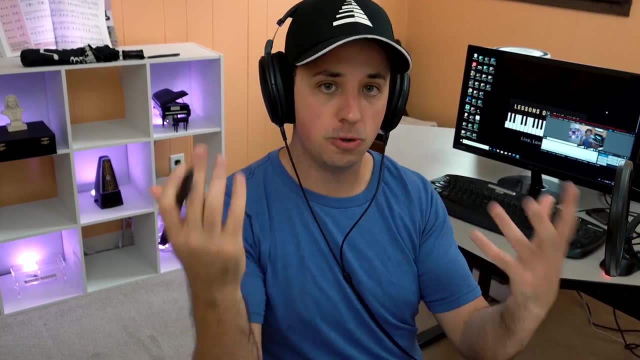 on each of the numbers that I have outlined. So when you're first doing these, you actually do wanna go through your music and chart out, like exactly how I did, using the subdivisions, drawing the lines to indicate how long to hold them for. So this one is super common. 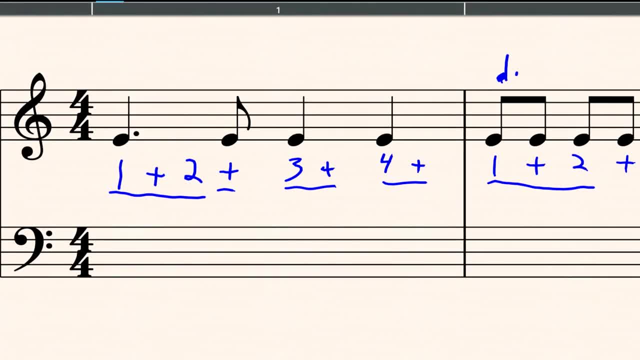 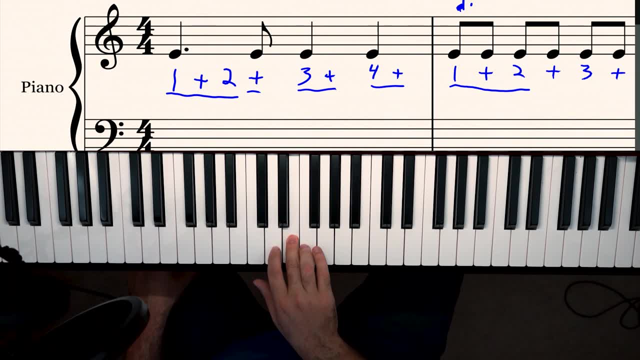 Students get this wrong for some reason all the time. It actually took me quite a long time to get the hang of it, So let's just do it together a couple times Ready: One and two And three and four, and One and two and three and four, and. 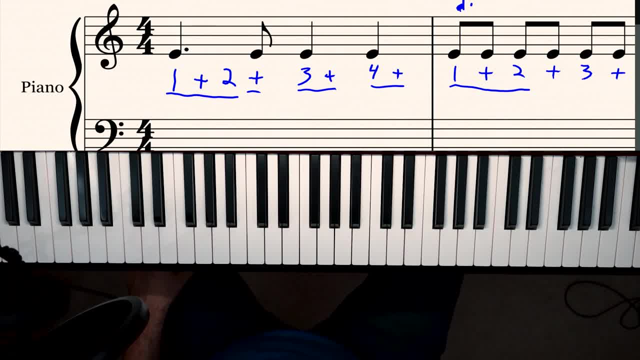 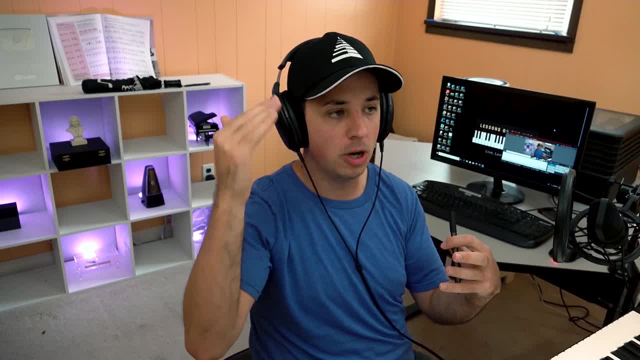 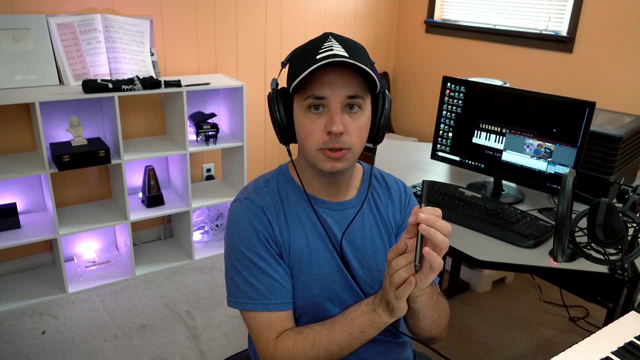 And then, beyond just counting it out, what I would do is I would actually start to kind of feel the rhythm in your body and start to kind of know, like just the sound of it, Bum, bum, bum, bum, bum. two and three, four. 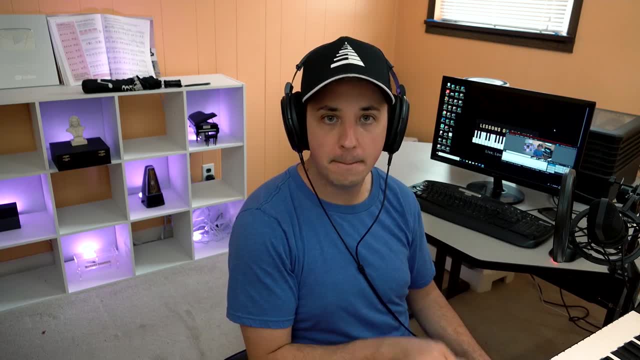 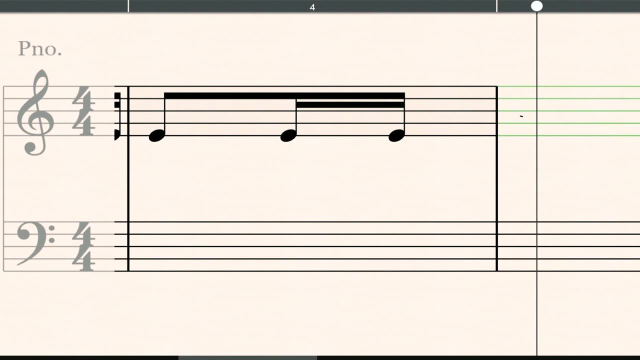 Bum, bum, bum, bum, bum. two and three, four. Bum, bum, bum, bum bum. two and three, four, Just like that. Okay, now we're gonna be talking about several patterns that have to do with eighth notes connected to 16th notes. 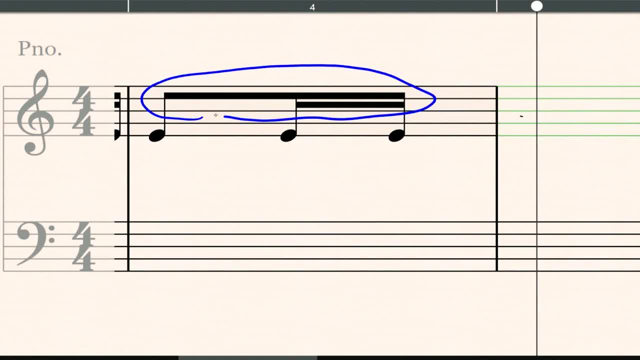 If you don't know already, when notes are beamed across like this, that tells you that together they're equal to one beat. Okay, to explain how to count these, what we're gonna do is we're actually gonna do kind of like what we did before with the eighth notes. 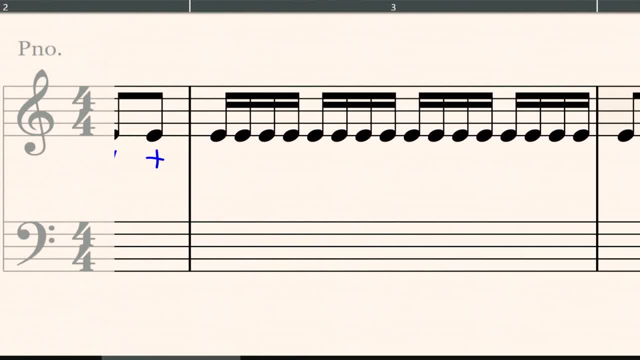 when I was showing you how you're splitting them up into one and two ands things like that. So what I'm gonna do is we now need to figure out. well, first I'm gonna show you that we still have all four beats. 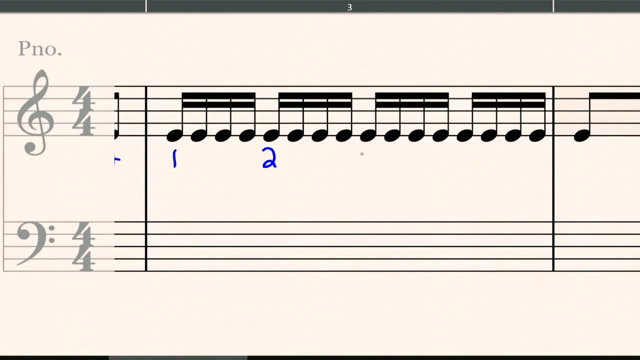 So each of these groupings of four are called the 16th. they're 16th notes. Oh, three comes after two. how about that? And then so we have our four beats. We still also have our ands, like before. 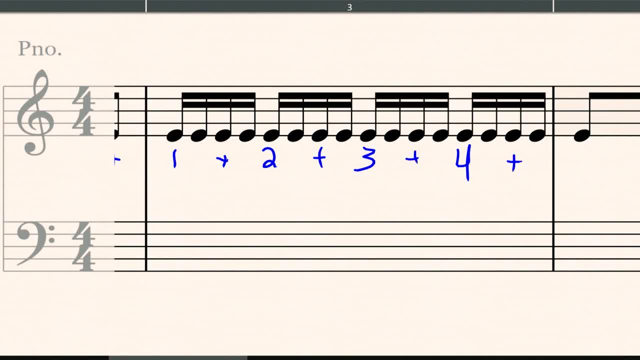 We're just putting them in the middle there. So therefore, we need some placeholders for these guys. So let's do that. Let me show you how that works. So we do that using the term. so you have beat one, and then you have e and a. 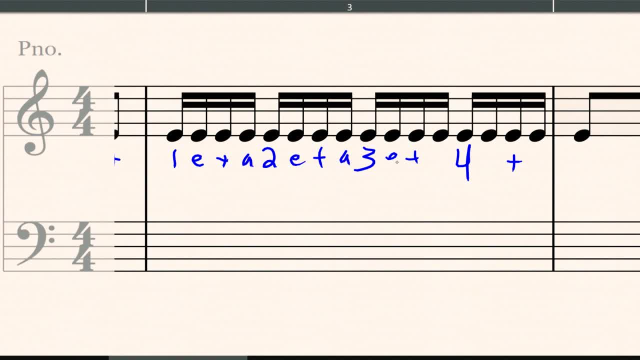 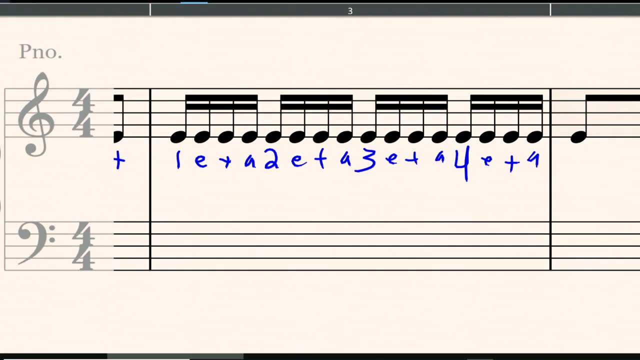 two e and a, three e and a four e and a. So therefore we are subdividing even further. We still have our one and two, and We have just broken them up now to be even faster. So back to the quarter notes. 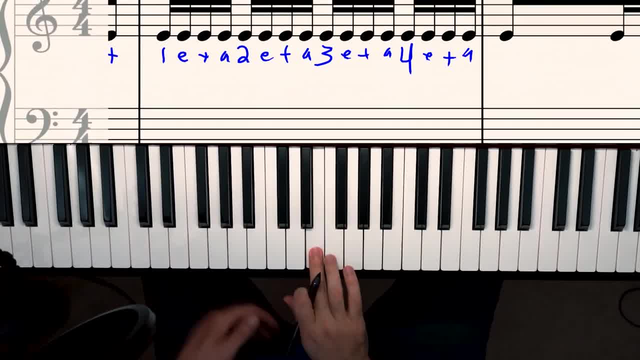 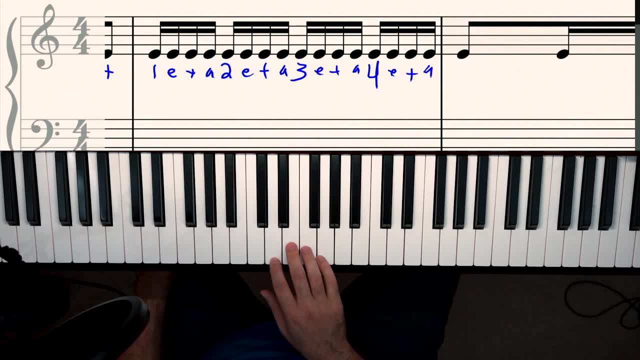 it would just be counted simply as one, two, three, four And then eighth notes. you play them twice as fast: One and two, and three and four and And then 16th notes are four times as fast, or twice as fast as the eighth notes. 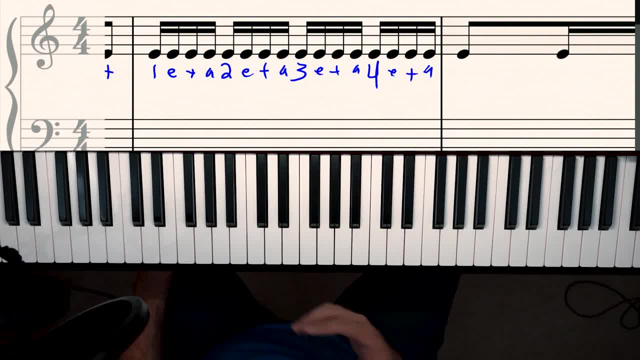 One e and a, two e and a, three e and a, four e and a. Takes a while to get used to, But keep in mind that this helps you figure out some of these patterns, just like how we did with the eighth notes to the dotted quarter note. 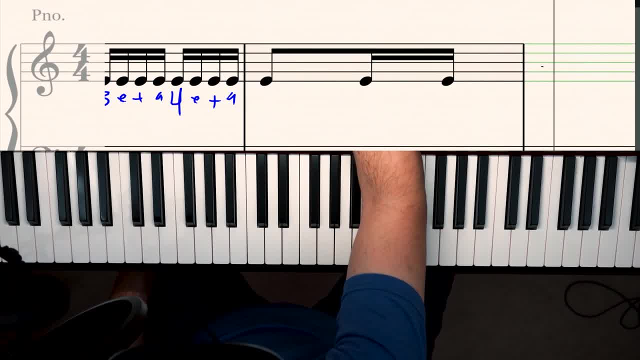 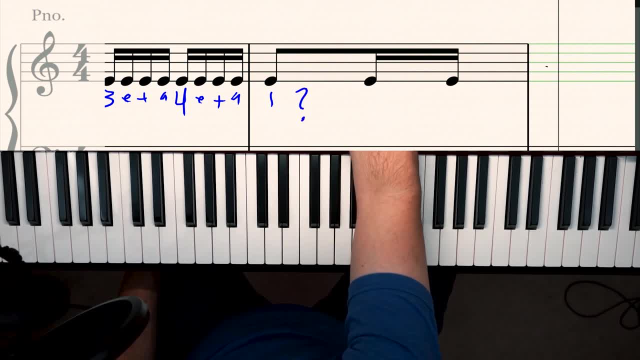 that we had before. So let me show you how this works. Obviously, we're gonna have beat one here right Now. the question is: all right, how long am I gonna hold that eighth note for? Well, we need to split up the beat. 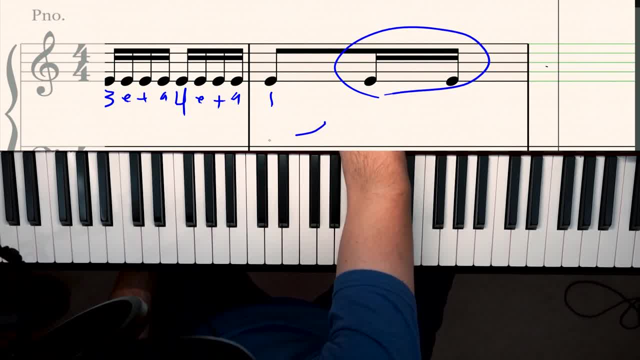 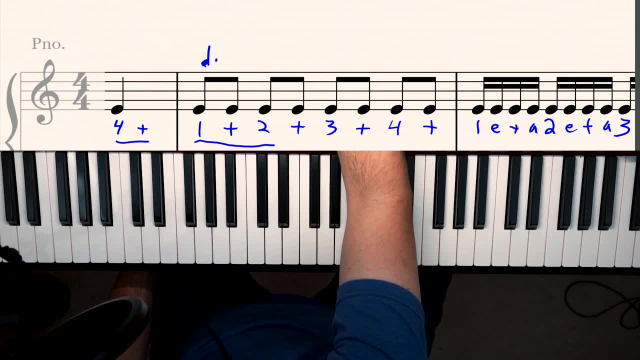 because whenever you're dealing with 16th notes in any fashion, you have to be subdividing into the one e and a two e and a type of formula. If you only have eighth notes in the piece, you can just kind of resort to the one and two and 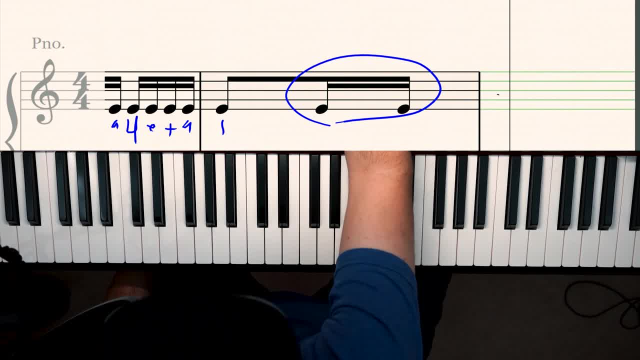 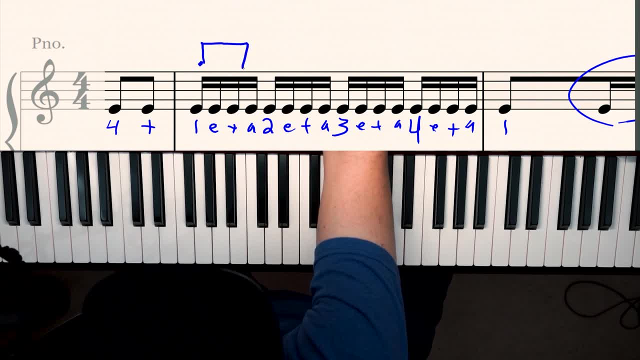 That's perfectly fine. Okay, so you have one and the eighth note now I'm gonna write up here. So this is what this is gonna look like. So if I had my eighth notes in place, they would take place on one, and 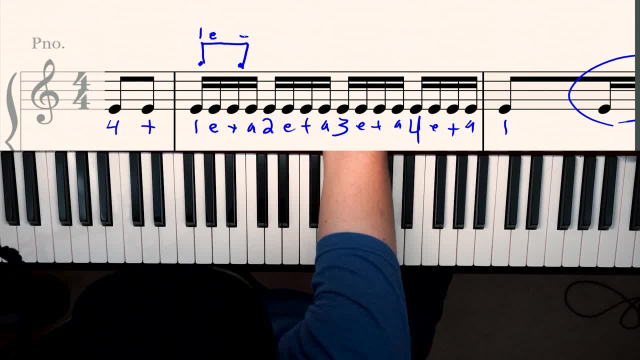 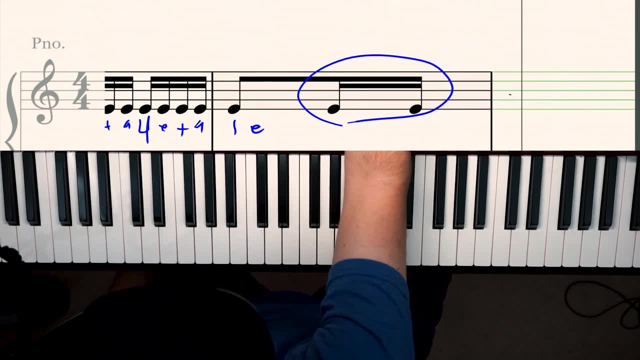 So really, this eighth note here takes up one e and this one is the one that takes up and a. So obviously, when we move this over here we have a single eighth note, So this is gonna be taking up one e. This means and occurs here: 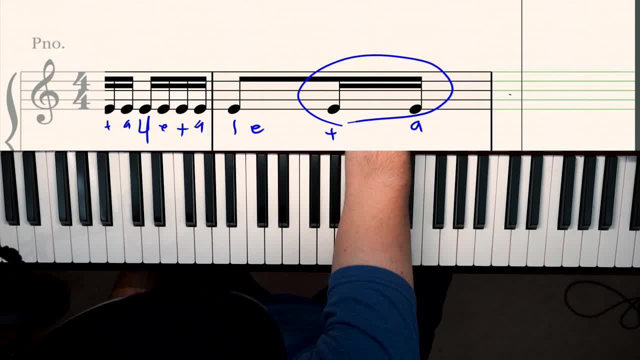 And then, since that's only a 16th note, our next syllable is gonna be a, So we're gonna be counting this as one e. So we're gonna be counting this as one e. So we're gonna be counting this as one e and a. 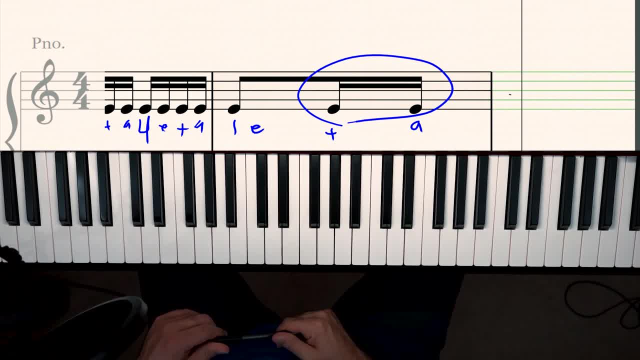 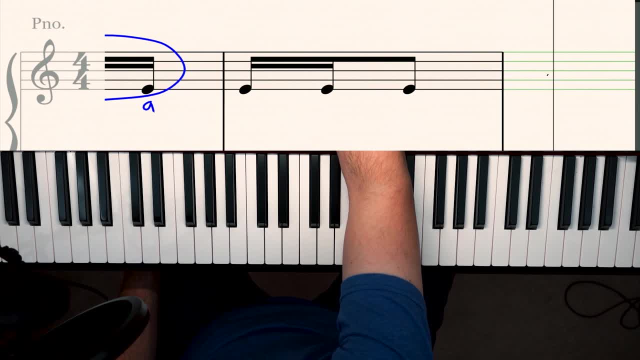 Just like that. All right, let me show you another pattern. Okay, so we had the eighth followed by two 16th, which we just did. Now we have two 16th followed by an eighth. So obviously we have 16th notes. 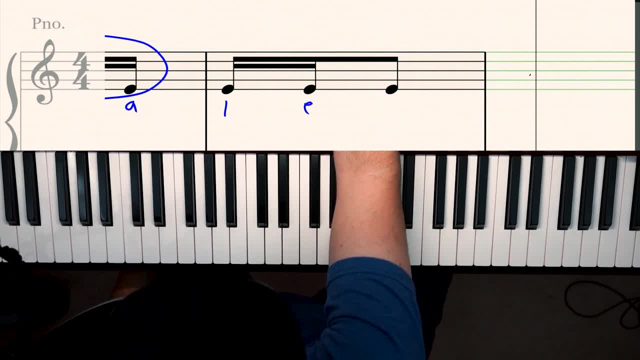 so we're splitting this up into one e right, And then, this time, the eighth note's on the end, so this is gonna get two of them right, Since you need two of these now, two quarters really to equal half of a beat. 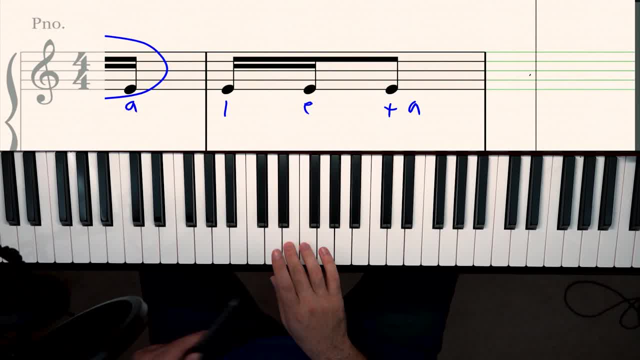 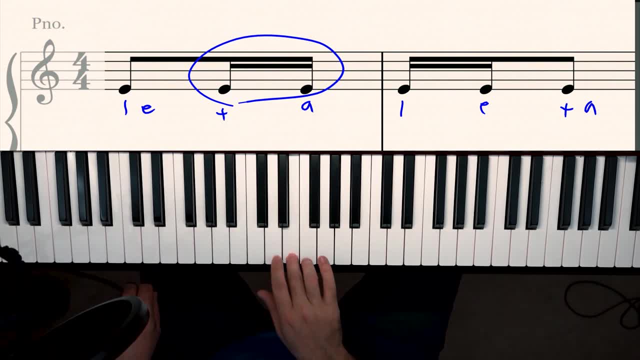 So that's the opposite. now It's gonna be counted as one e and a. The first one I'm gonna count them both back to back is one e and a, And then the next one is one e and a, Just like that. 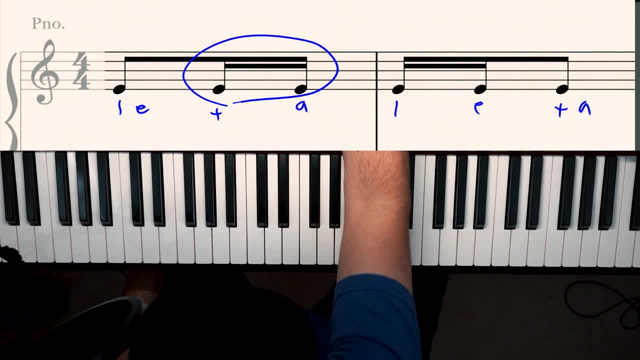 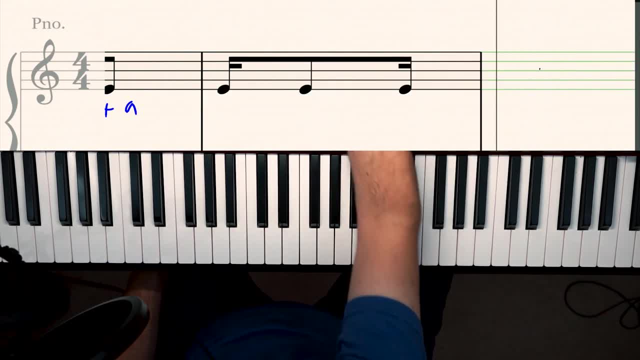 And we'll do a little practice kind of combining them all into the same measure as we go along. All right, let me show you one more combination of eighth, 16th pattern. Okay, we have a new pattern, We got a 16th here. 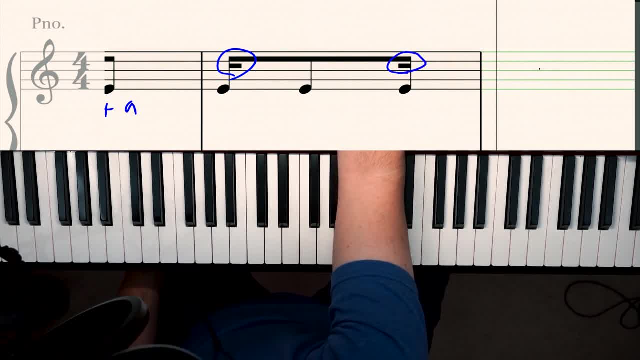 You can always tell by the double fourth. You can always tell by the double flag: 16th here. So therefore we have to be using our one e andas right. So whenever you have a 16th note like this first note, 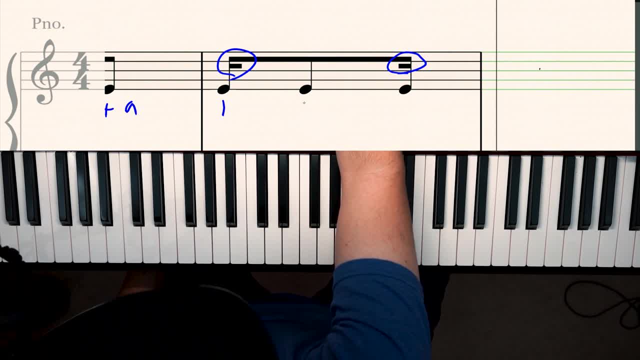 it's just gonna take up one of the syllables, So one, and then the next syllable has to be on that next note. You know it can't take up any more space than that. Now, this is an eighth note. 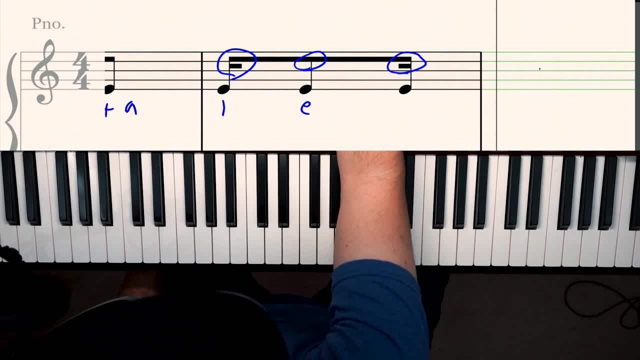 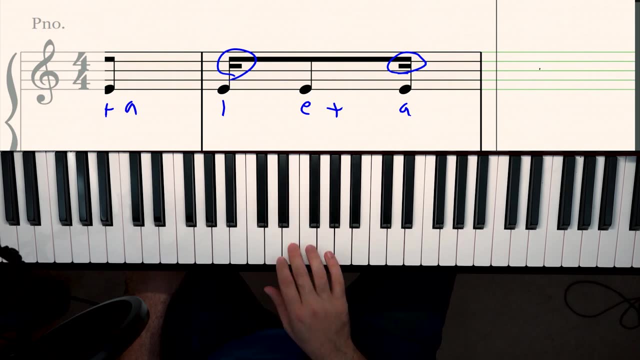 You can tell, because the beam connecting across only has a single flag up top, not two of them like the others. So this is gonna take up e and, and then you have uh right here. So this one's gonna be counted as one: e and uh. 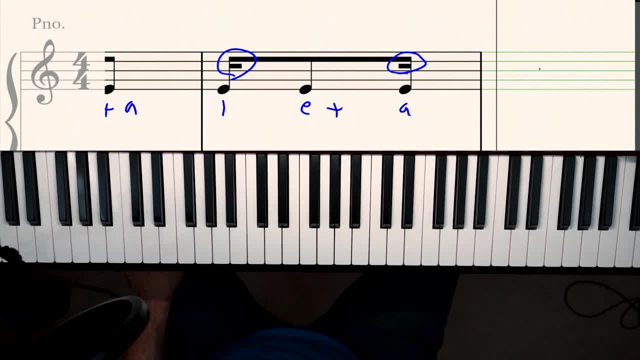 One e and uh, And just like the dotted quarter eighth rhythm. I told you before you wanna get the feeling of all these, So, even without you, wanna count them first, but then, after a while, you wanna just get the feeling of it. 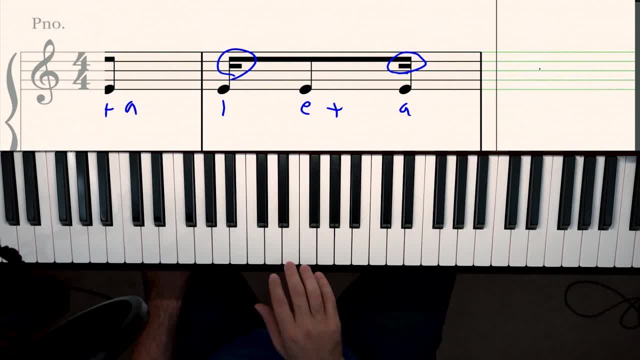 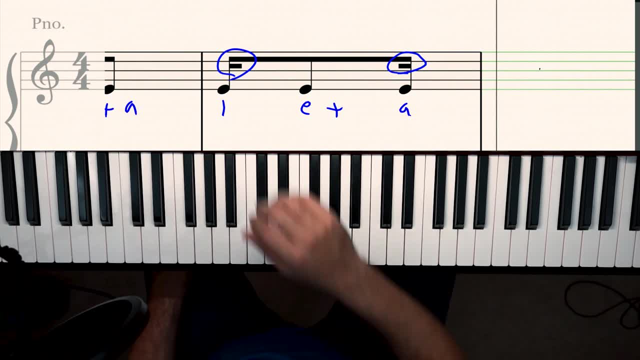 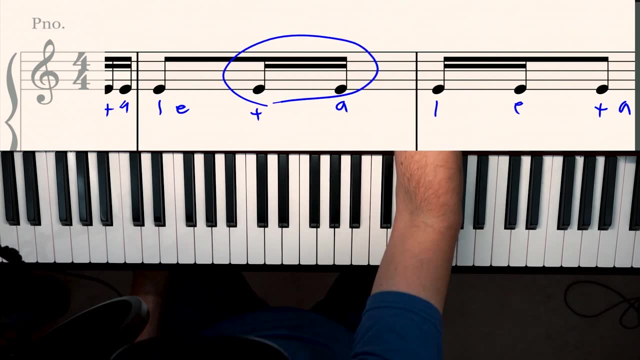 One e and uh, one e and uh, one e and uh, and then Bum, bum, bum, just like that. And then same thing with these I kinda forgot to mention. This one is bum, bum, bum, or one e and uh, just like that. 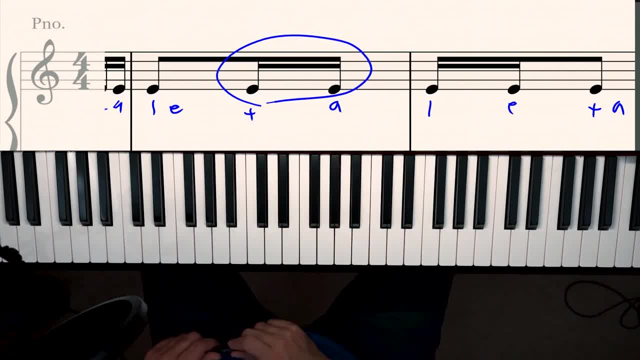 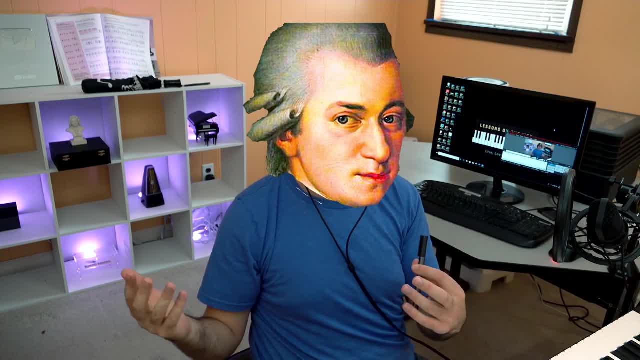 And this one is one e and uh. All right, now let's see how good you are. We're gonna kinda combine a lot of these eighth, 16th patterns together, see if you really get it, and then we'll move on to something else. 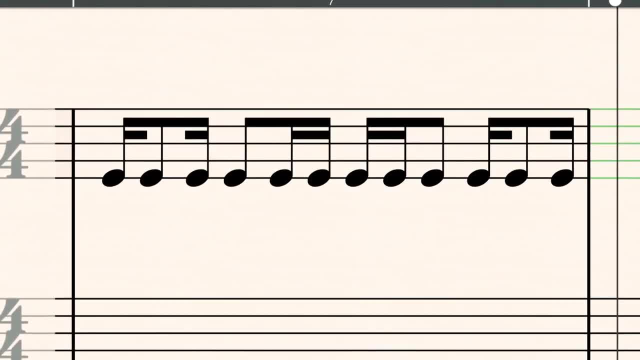 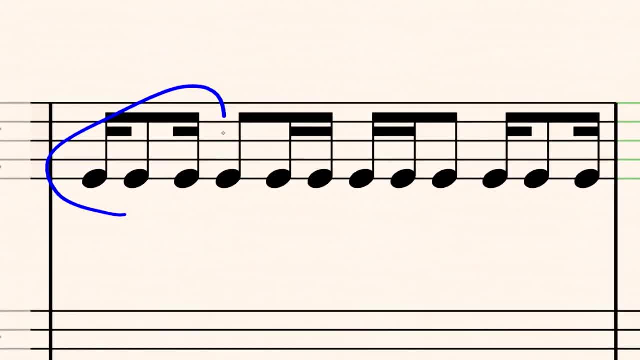 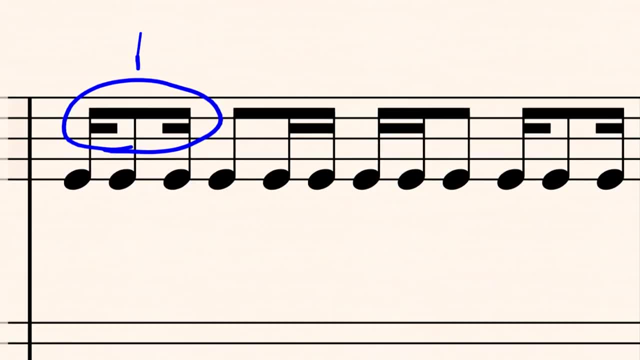 Just kidding, It's not nonsense. Okay, so we got our first grouping here And, by the way, they're all beamed together. So what does this beaming mean? if they're all beamed together, That means that this equals one beat. 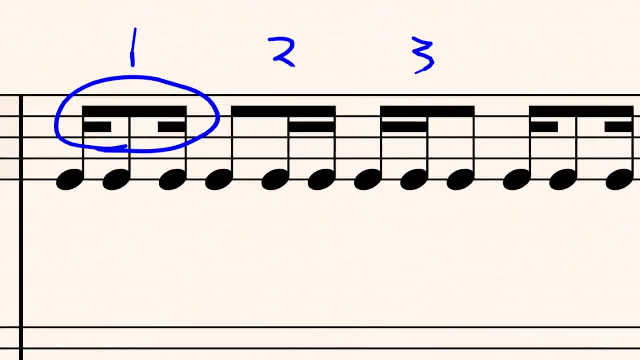 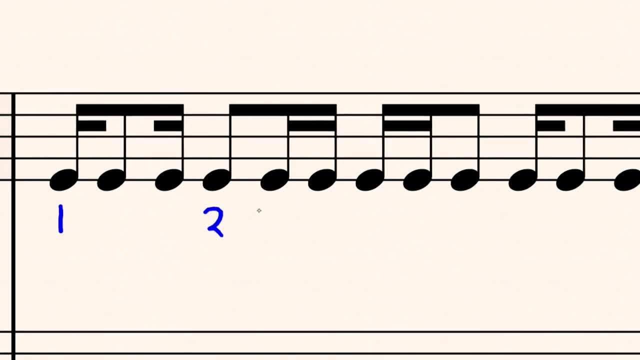 You know the next one's, two, three, four. So we know that we have our four beats there, because when they beam them together that's one beat. So you have beat one here, obviously in that first grouping. So let's just write out: yeah, where the three beats. 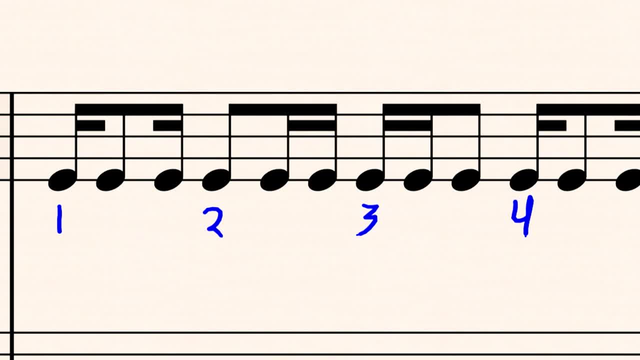 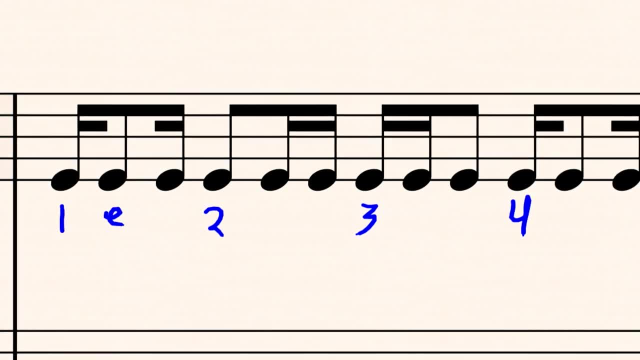 four beats, sorry will occur. So here we go. We have a 16th note right here, So this can only take up one out of the four cymbals of the one E andas, So this has to take up E this next one. 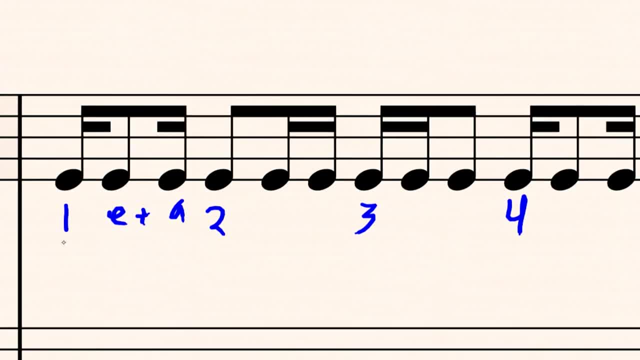 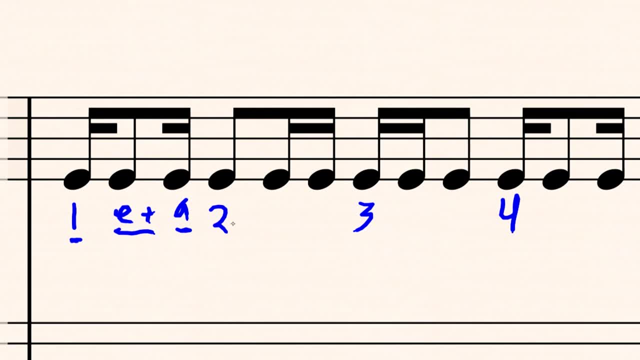 That's an eighth note. right there, E and a, And then draw the lines if you need to make sure you know where they're hitting. And then on the second one you have two, but this is an eighth note, So this is gonna be taking up two E. 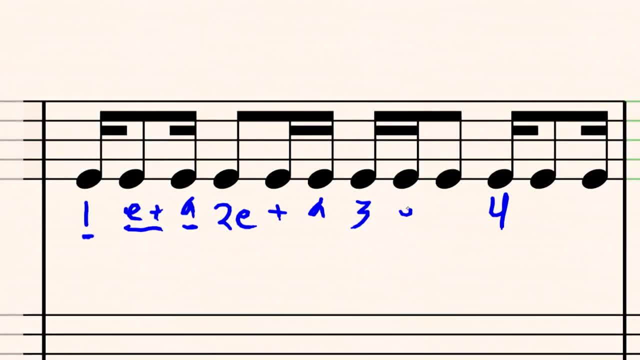 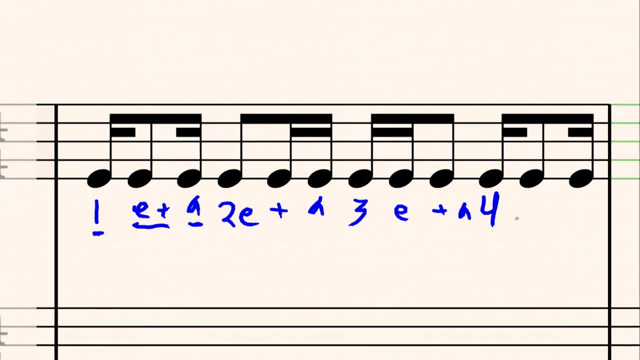 And then you have anda. This one is three E because they're 16th notes. This eighth note's gonna be anda, And then the last one is the same as the first one. So you got four E and a, And let me just draw the little lines here. 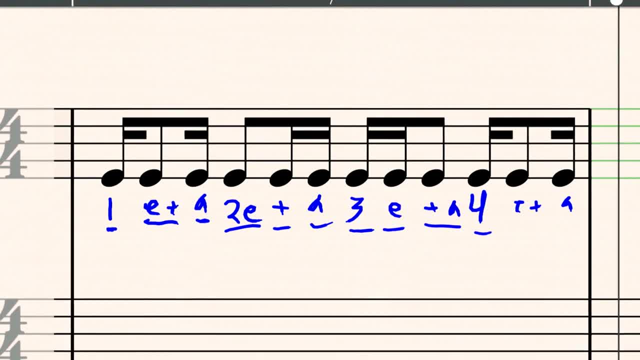 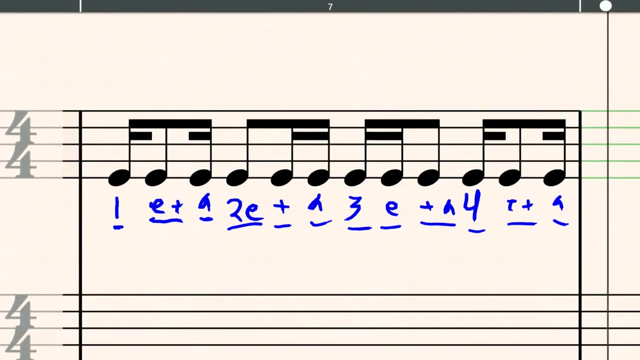 They do help me at least, And then this might be confusing at first, but it does get easier and easier. One way you can check to see whether you are correct or not is if you have all four syllables of each beat written out. 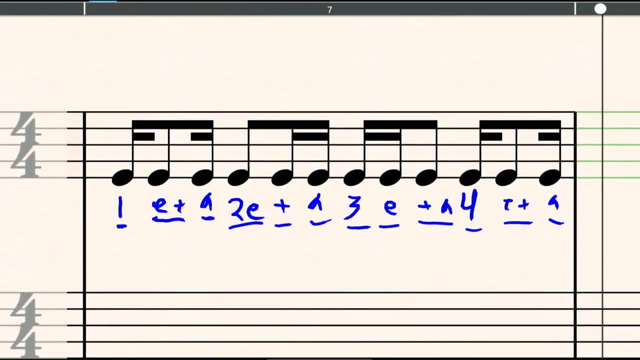 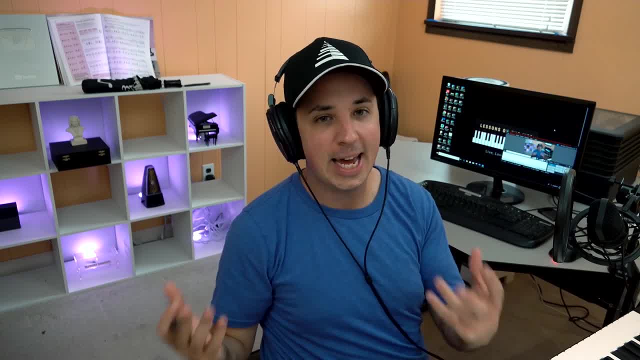 Because if you're missing any or you wind up at the end and you don't have enough notes left, then you know Your notes. I know you goofed somewhere, so then you gotta kinda go back and check. It is gonna happen to you, especially at first. 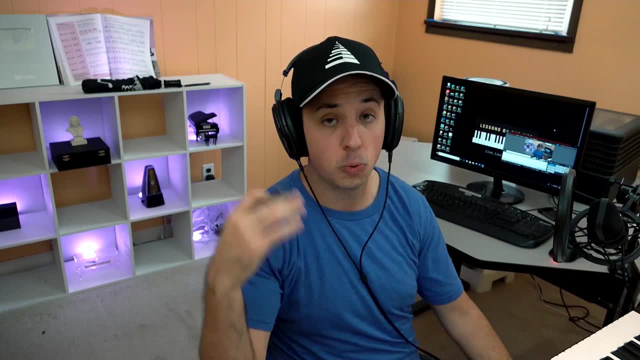 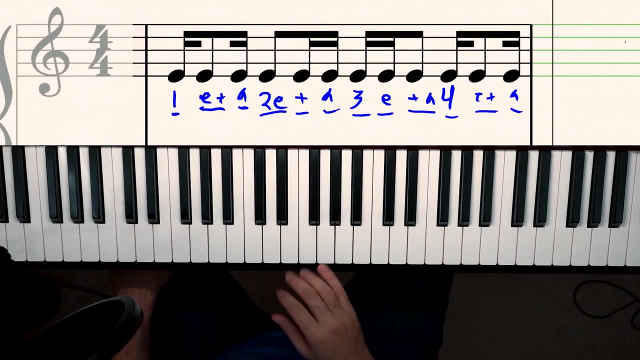 It took me quite a while to get used to this, but make sure you keep practicing it because you will see these patterns quite a lot. All right, let me count these out now. So when you're actually playing them, you wanna play them nice and slow. 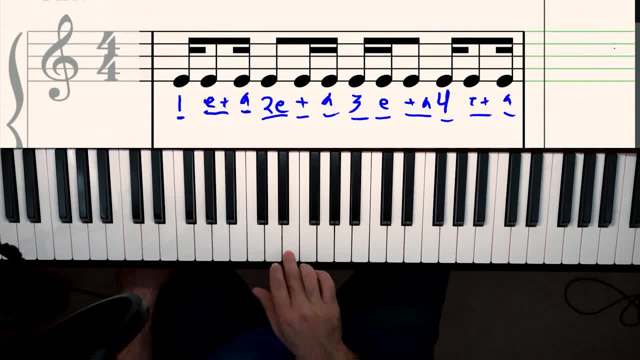 So here we go: One E and uh, two E and uh, three E and uh, four E and uh. So I'm pretty good at it. It might take you a couple times to count through. 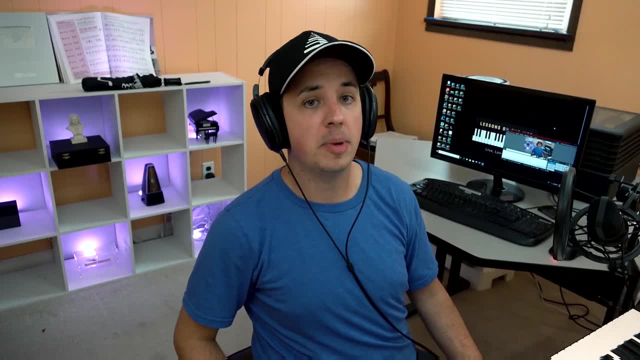 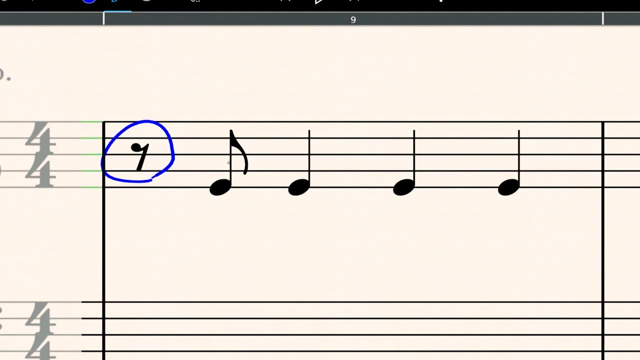 All right, let me show you another fundamental rhythm pattern that students often get wrong. Okay, we're doing a simple one Now. this is an eighth rest. It's the same as the eighth note, except you don't play. Make sense. 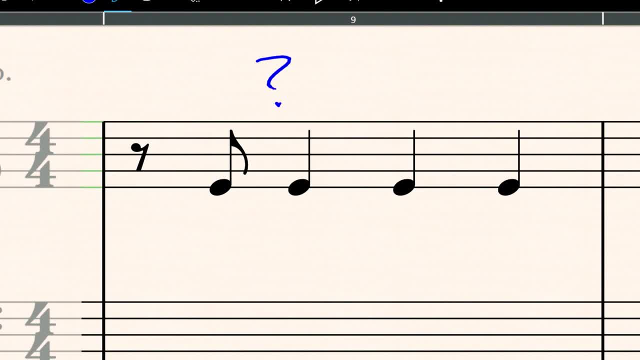 So do we have any 16th notes in this measure? No, we do not. I don't see any double flags or anything that would look like that, So we only need to really count out the one and two ands. So what I would do is: here we have an eighth rest. 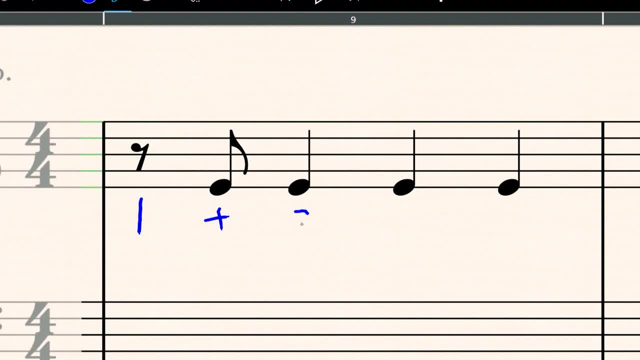 So it's gonna take up one- This is the other half of one- And then two, three, four. However, I would still be counting these, the ands in between. That will just make sure that you're playing them as consistently as possible. 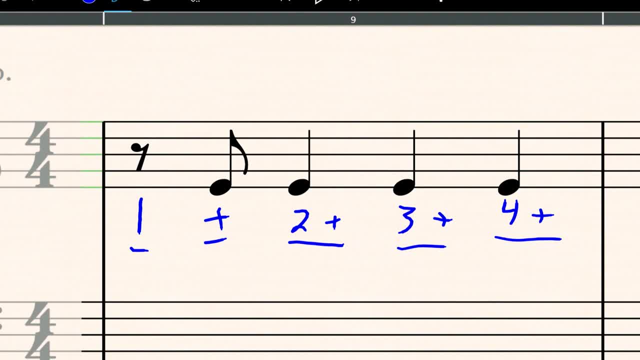 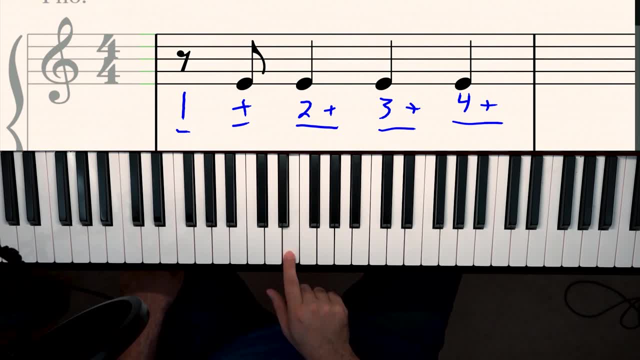 So this I would just call the eighth rest, eighth note pattern. So here we go. This is how you're gonna count this, nice and slow. So you're gonna go one and two and three and four, and one and two and three and four. 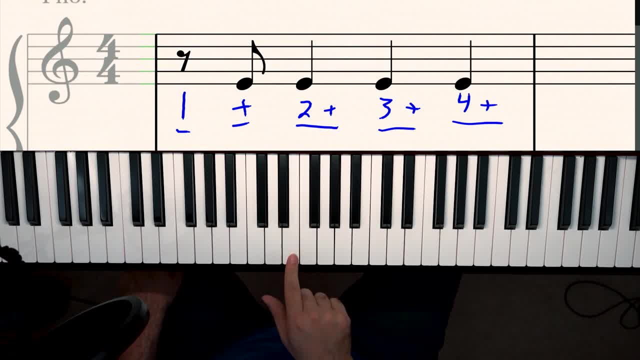 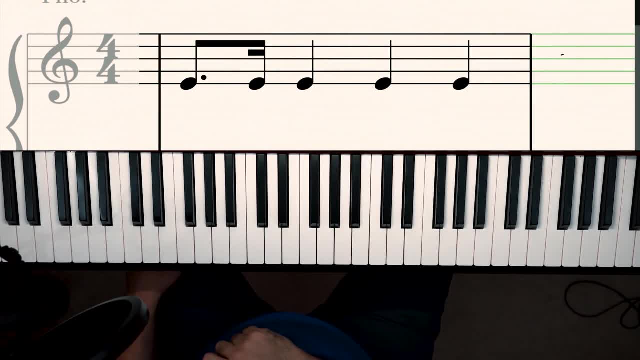 and one and two and three and four, and just to give you some feel for how that's gonna go, All right on to the next one. Okay, the next rhythm I'm gonna teach you is the dotted eighth 16th rhythm. 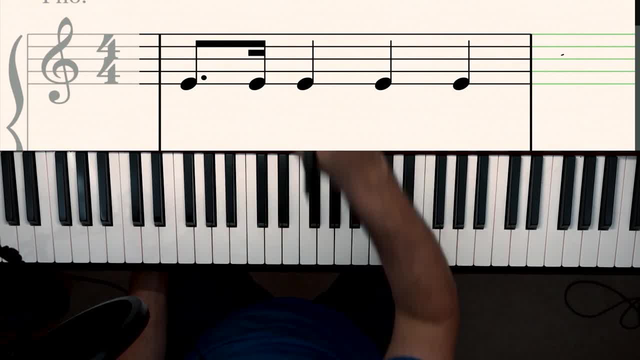 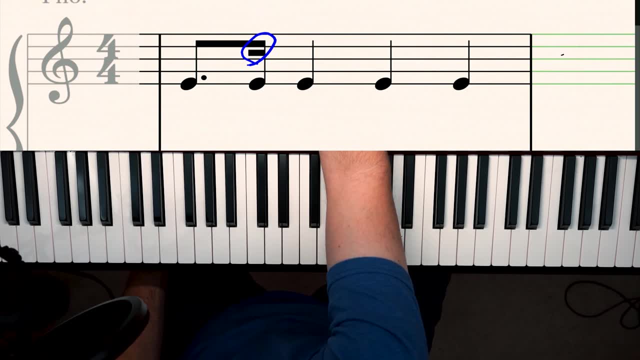 So here we have a dotted eighth note, And the first question I actually wanna ask you is: are there any 16th notes in this measure? The answer is yes. you can identify that one right there And that tells you you're gonna be subdividing. 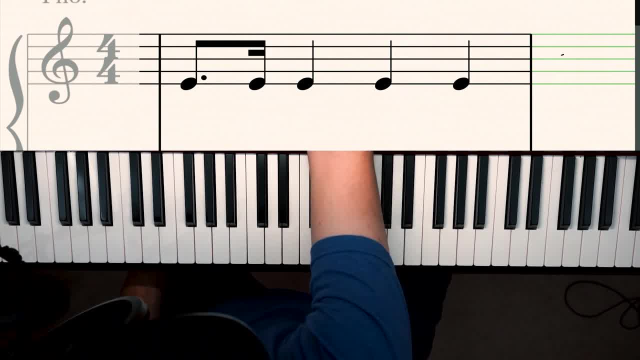 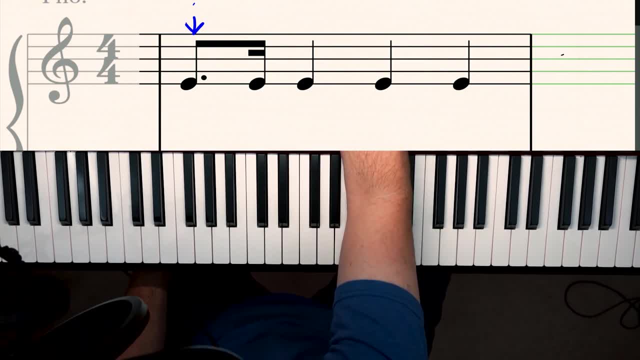 into the one e and a two e and a kind of format. So the real question is, which is kind of confusing, is how many beats in that dotted eighth note? Well, if you remember the dot, I mentioned this actually in the other lesson I did. 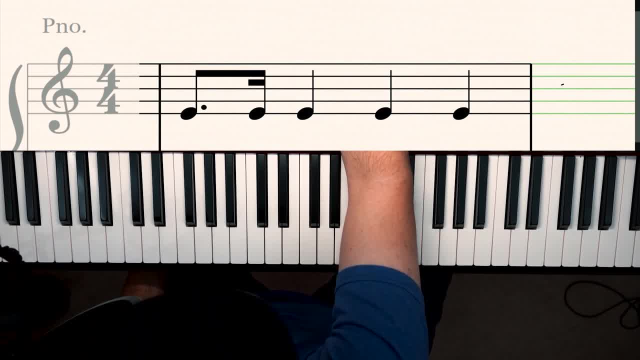 that I told you to watch and that the dot adds half of the note's value to itself. So here we have an eighth note and that's worth half of a beat, And here with the dot, we're adding half of a half. 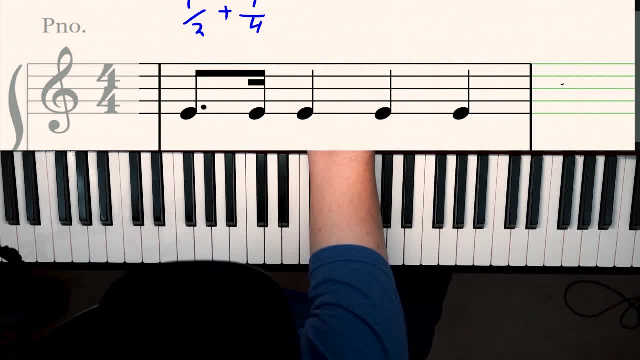 which is a quarter, which, as you remember from math, that you're gonna have to convert this one to two over four, So two over four plus one over four. So therefore the dotted eighth is gonna get three quarters of a beat. 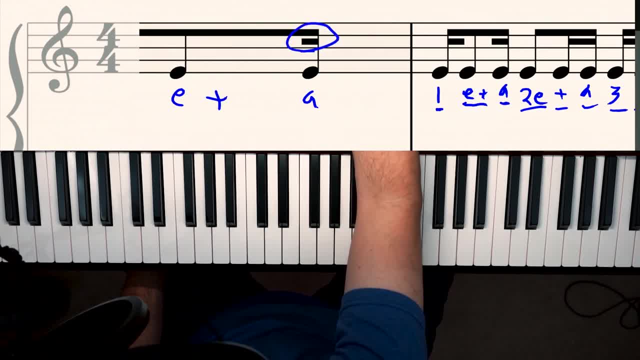 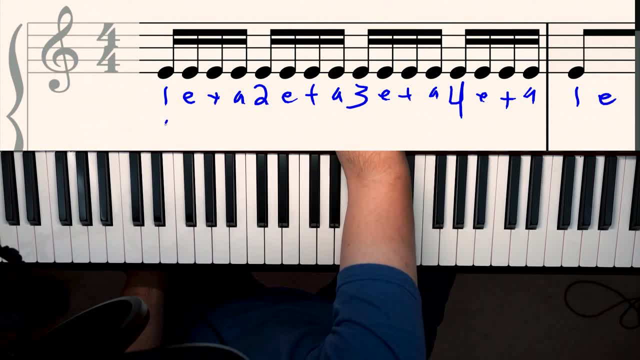 So when we go back to our 16th notes, where are they? they're way back here. there we go, And I'm gonna get rid of this now. So now, when you're doing the one e and us, each of those now represents a quarter of a beat. 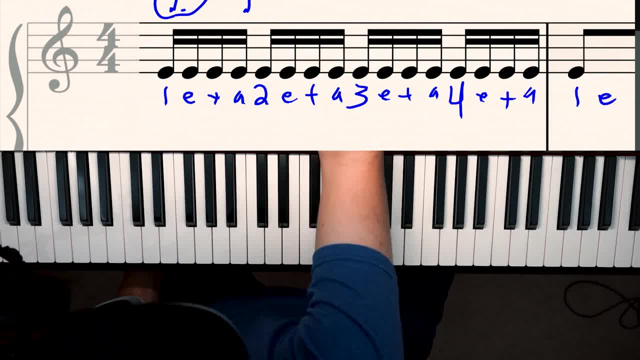 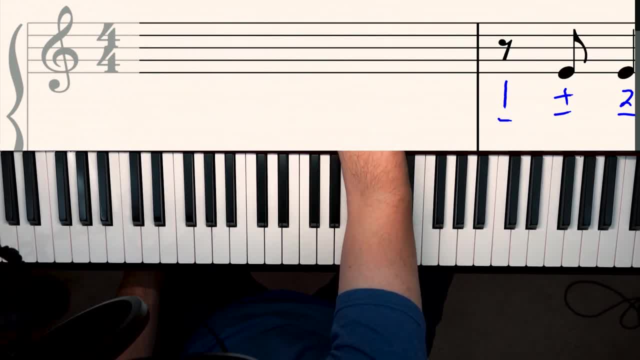 So we need three quarters of a beat. So therefore, our dotted eighth is gonna take up one e, and since each of those represents a quarter of a beat, So let's shift it over and apply that to what we're doing here, And here we have beat one, obviously. 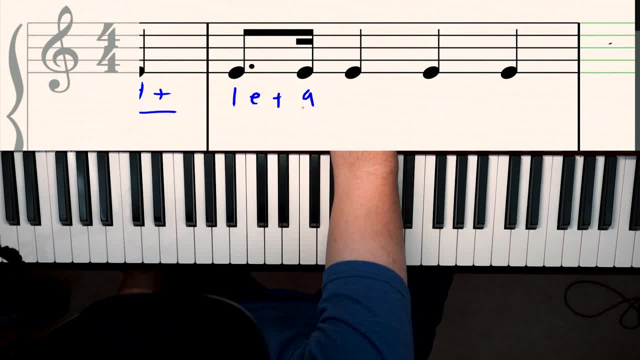 And remember I said it's gonna take up one e and This is gonna be on uh. So that checks out, right, because that makes one complete beat and those are beamed together And then you wanna count out the rest of the beats. 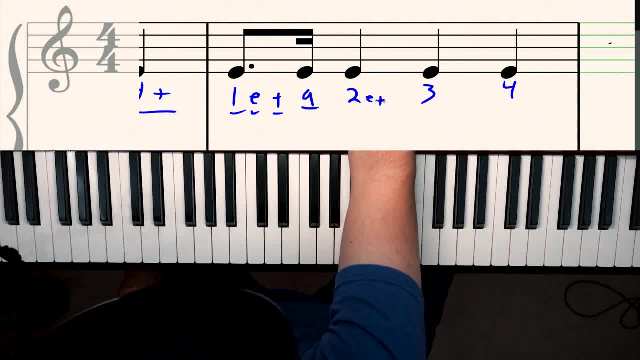 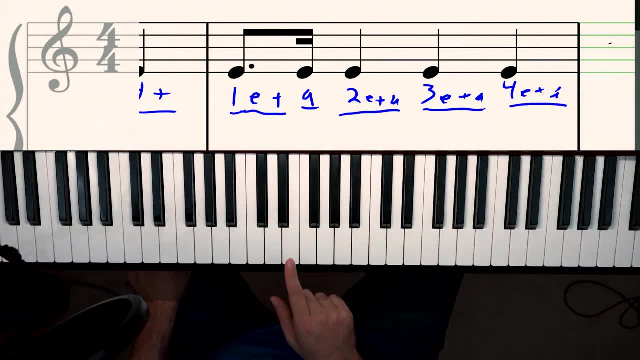 So I just like to write the numbers first, But you still wanna be counting the e and-as, as I like to call them, just like that. So here we go, I'm going to play this. one One e and uh. two e and uh. 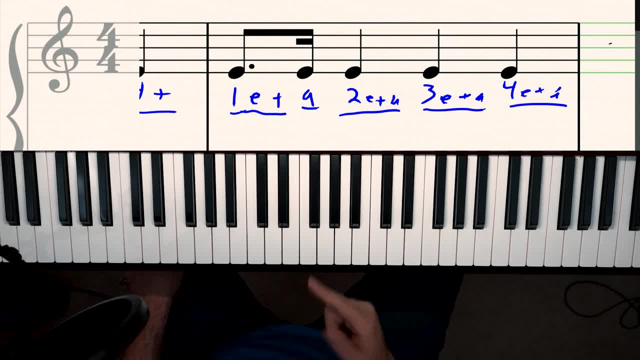 three e and uh four e and uh One e and uh two e and uh three e and uh four e and uh One e and uh two e and uh three e and uh four e and uh. Once again, one e and uh two e and uh. 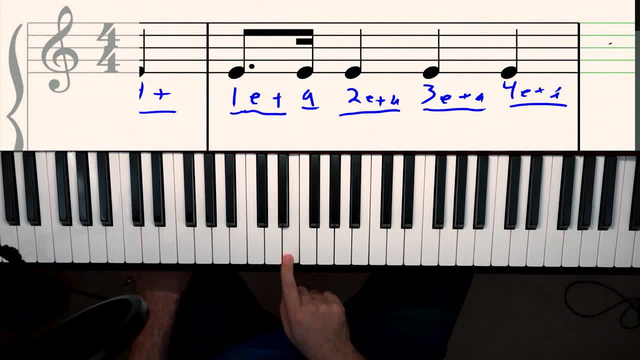 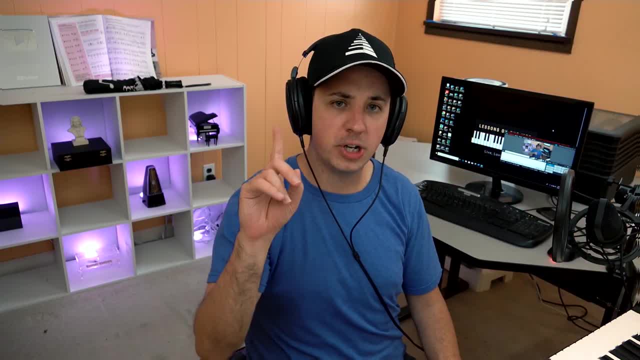 three e and uh. four e and uh. If you're liking this lesson, make sure you smash that like button. Really helps me out. You need some more practice on your rhythm, of course, so you wanna check out this lesson right here. 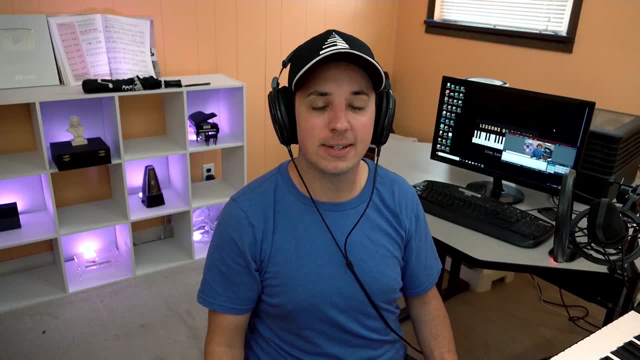 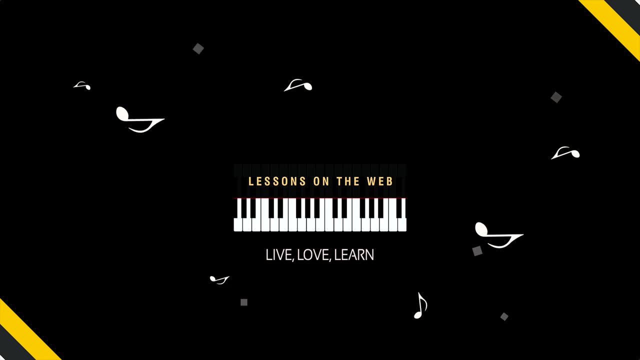 And that's been your piano teacher, Tim here. Thanks for coming by today and I'll see you- yes, you- in the next lesson. Captions by GetTranscribedcom. 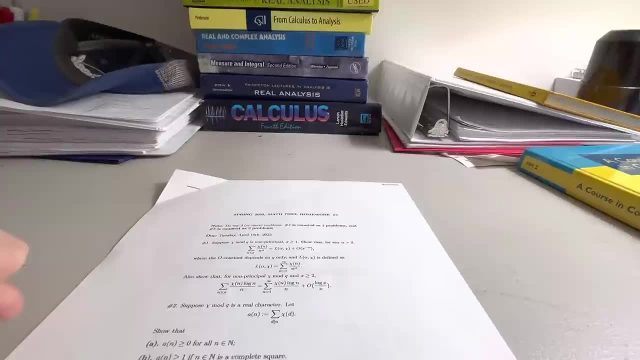 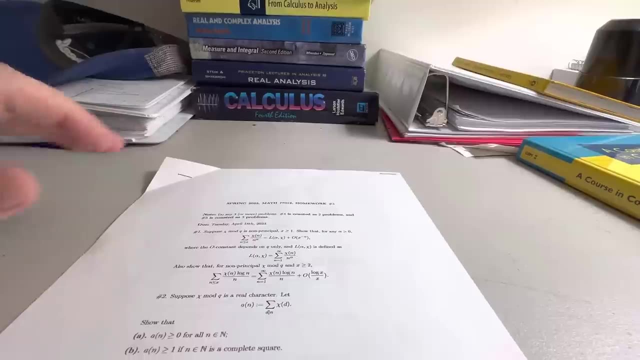 I am taking three classes this semester. Probability Theory is the one I think I've talked about the most, and the other being Convex Geometry, or the class is really called Problems and Uniqueness, but I call it Convex Geometry. And the third one, which I've rarely 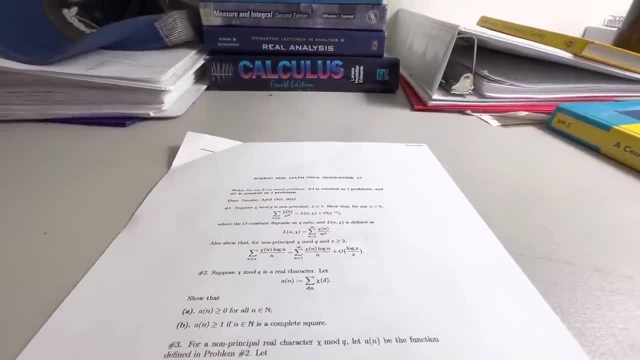 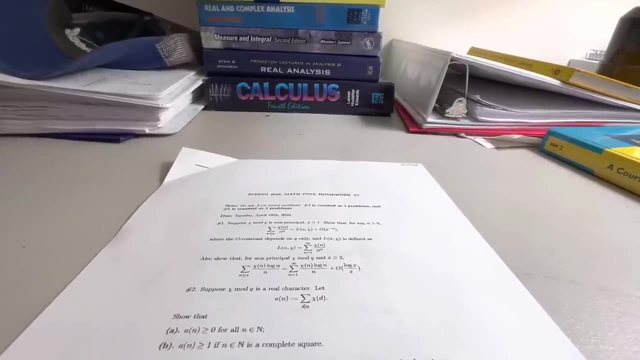 spoken about- I don't even know if I've really mentioned it all that much- is Analytic Number Theory. The reason I don't talk about it very much is because we don't get a whole lot of assignments in the class, so we just kind of show up, take notes and that's it. There's no real 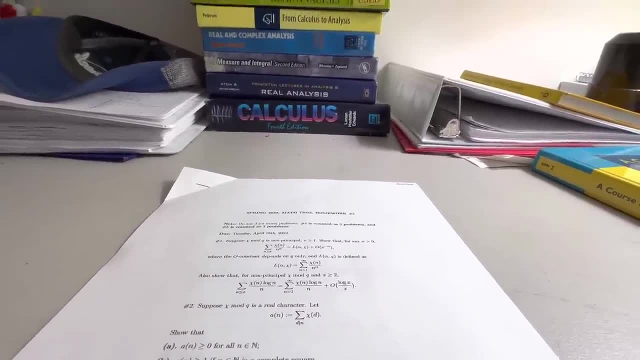 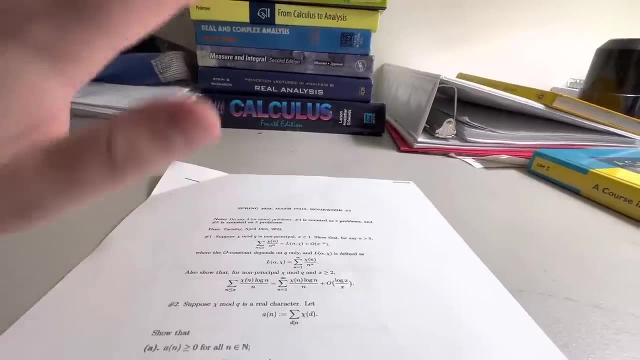 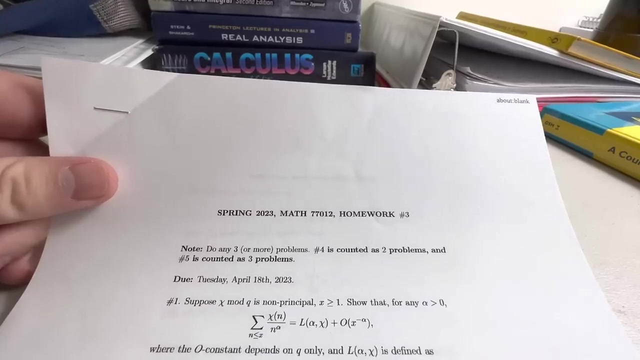 tests in that class and we're graded based on homework assignments, And yesterday we were given our very first homework assignment and I printed- well, okay, not the very first, I don't know why- I said that The third homework assignment is given here. So this is three pages, but as you